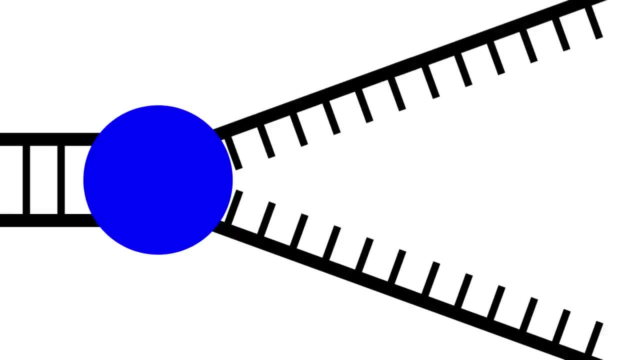 With the strands separate, we can begin to copy each one, but the enzyme that copies the strand needs a place to start. so an enzyme called primase will anneal an RNA that will be a DNA polymer at a specific location to kickstart the replication. This primer is: 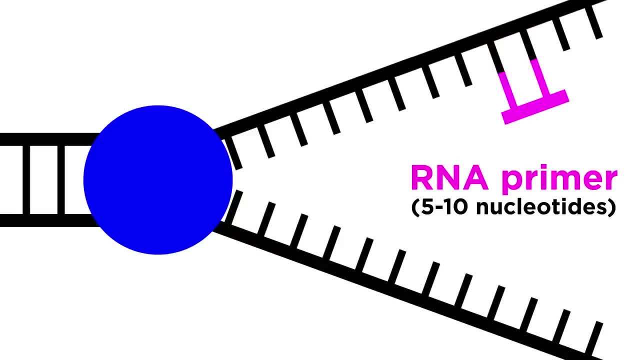 about 5 to 10 nucleotides long. Then another enzyme called DNAPolymerase III binds to the primer and begins to generate a whole new complementary strand, adding nucleotides to the new chain that was initiated by the primer. Nucleotides enter the enzyme's active site. 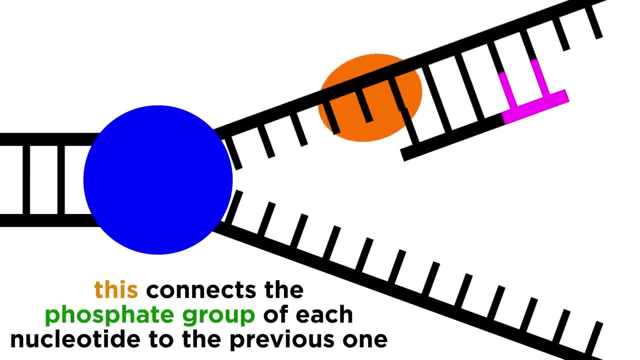 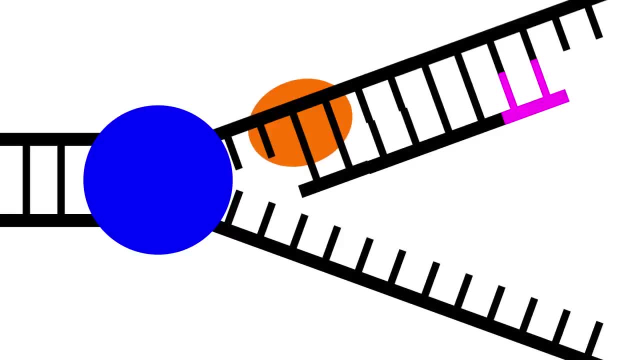 and polymerase catalyzes formation of the phosphodiester bond that joins each new nucleotide as it is added to the complementary strand. This process will be different for each strand, because polymerase will always add nucleotides to the three-prime end of the existing strand. not the five-prime end and the strands are anti-parallel, so the direction of replication must be in opposite directions for the opposing strands. On the leading strand, DNA replication moves along with the replication fork, continuously synthesizing DNA. But on the lagging strand, polymerase has to go one chunk at a time. as new template, 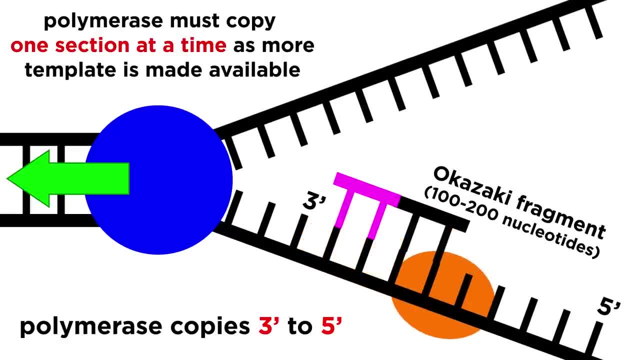 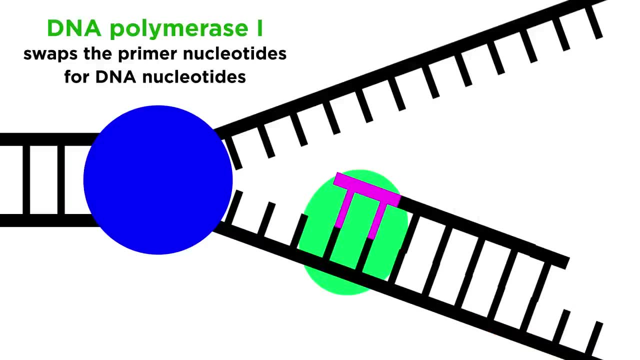 is made available. These chunks are called Okazaki fragments and they are around 100 to 200 nucleotides long. Each one will require its own primer in order for polymerase to bind and copy the new fragment. After each fragment is synthesized, DNA polymerase will: 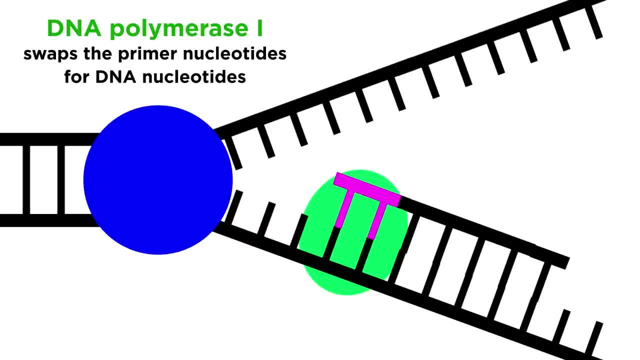 go through and replace the RNA nucleotide from the primer with DNA nucleotides to make sure it's DNA all the way through. Lastly, because polymerase can't join the last nucleotide of one fragment to the first nucleotide of another, a separate enzyme called ligase has 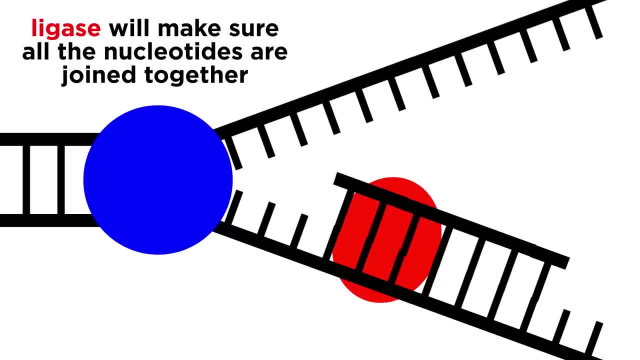 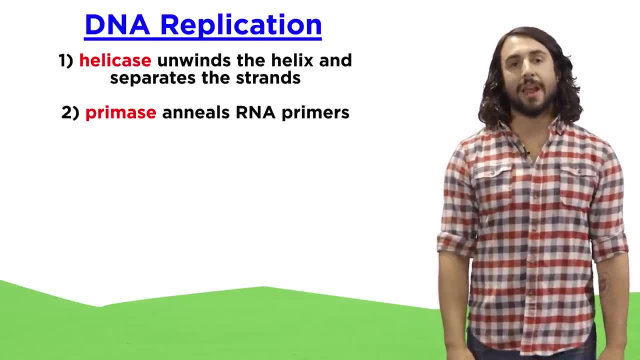 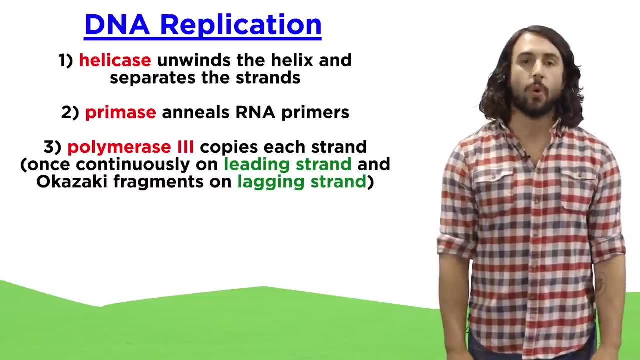 to go through and make sure everything is connected. So to summarize: helicase unwinds and separates the DNA into two strands. Primase anneals, primers, things off, and polymerase III copies each strand. On the leading strand. we need just one primer and everything goes continuously. 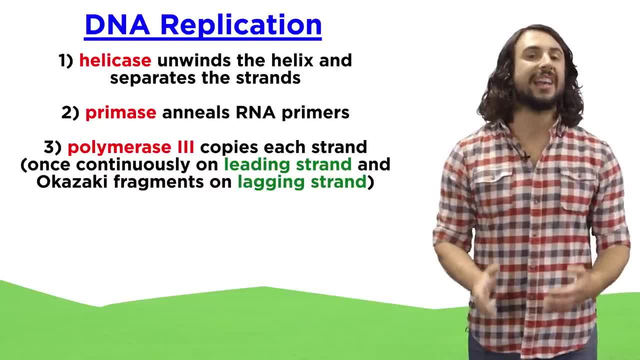 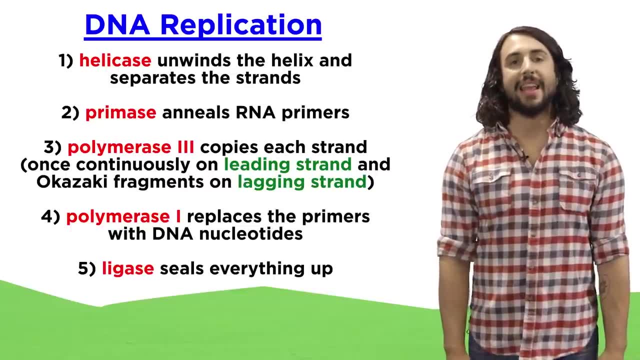 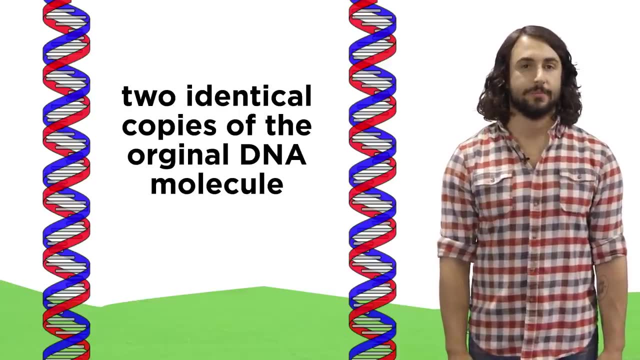 On the lagging strand. we need a primer for each Okazaki fragment. Then polymerase- I replaces the primers with DNA nucleotides- and ligase seals everything up. Boom- two identical copies of the original DNA molecule. This whole process which is happening in billions of cells in your body at this very 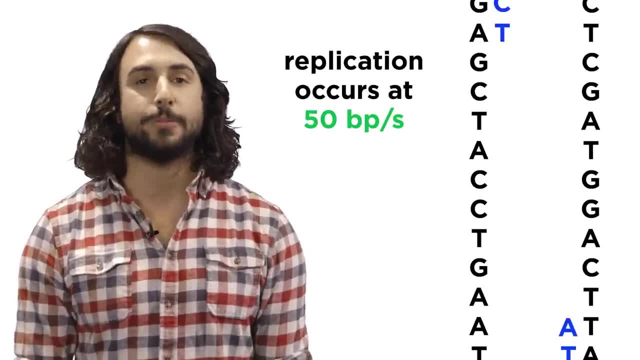 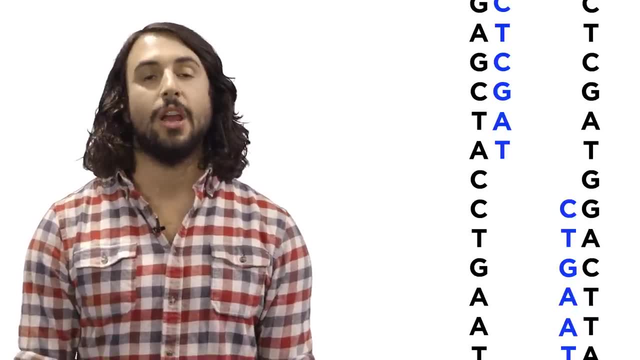 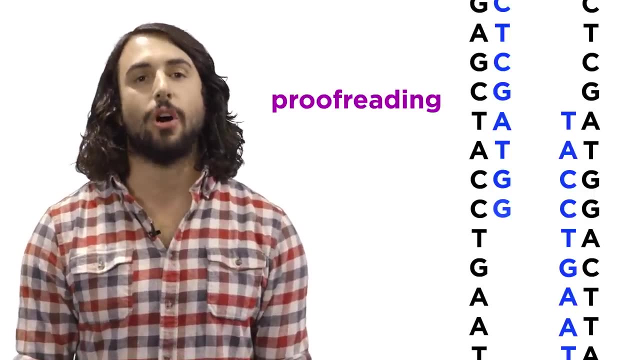 moment goes very fast: about fifty base pairs per second. Moreover, polymerase is very good at getting the code right. it almost always puts the correct base across from the template strand, and when it makes a mistake it can usually backtrack and correct it in a process called proofreading. 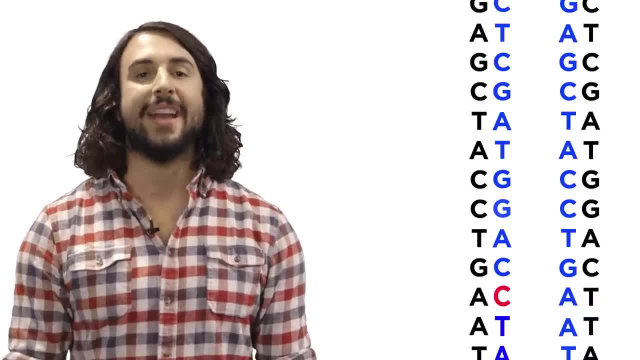 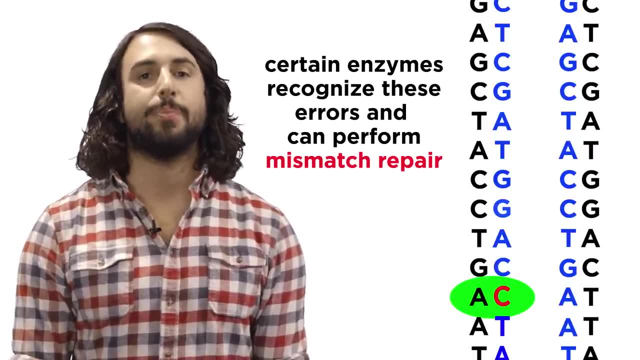 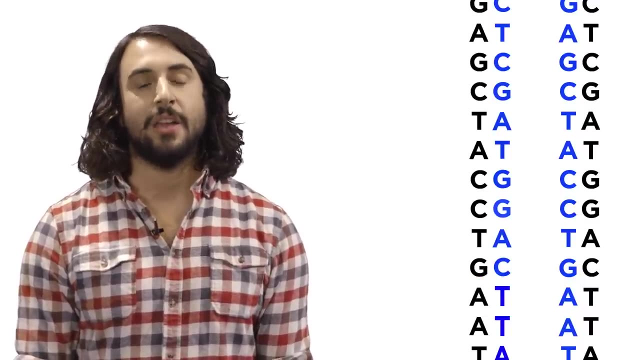 Even with this, around one in every ten billion base pairs an error ends up in the process. Luckily, there are enzymes that can recognize these errors and perform mismatch repair, swapping out the incorrect base for the correct one, just like other enzymes that repair damage. 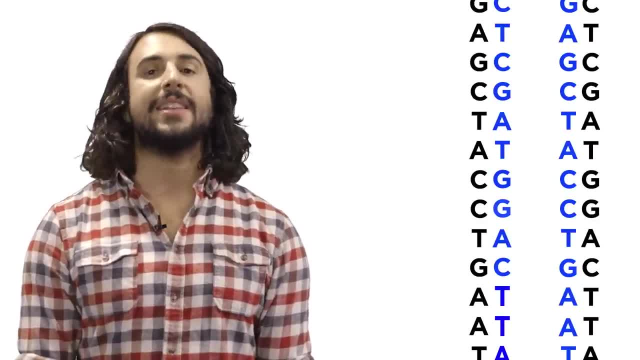 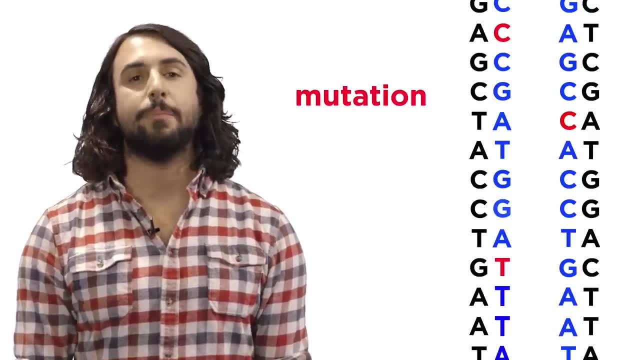 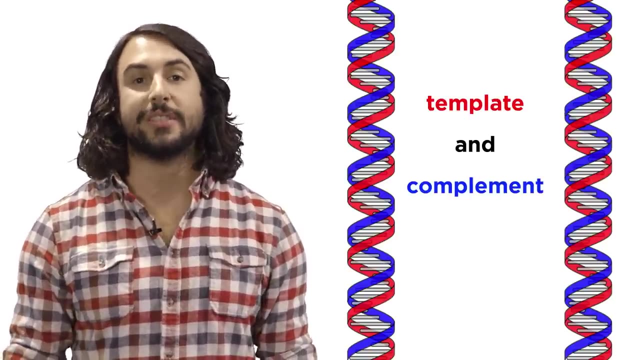 caused by external sources. These enzymes minimize the possibility of mutation, and we will learn about them later. But, as we said, polymerase almost always gets it right. in this way, each strand in the double-helix acts as the template for its complement, and we end up with two identical copies of all. 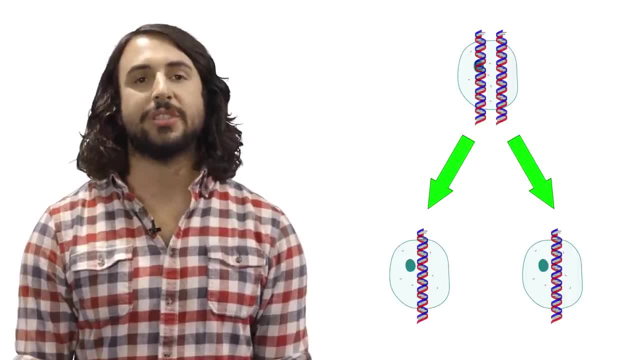 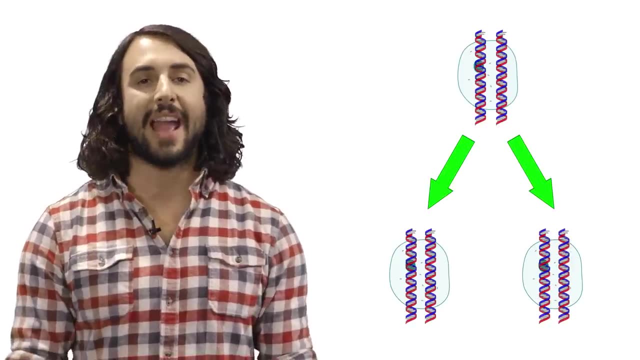 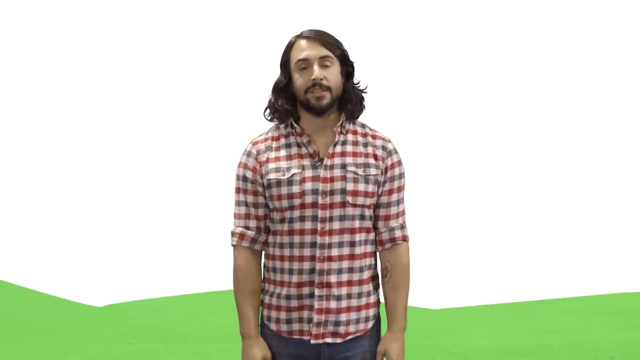 the genetic material. When a cell divides, each new cell retains one of these copies, and when the cell cycle gets to a certain point, these new cells go about copying everything again to be ready for another division when the time comes. Thanks for watching, guys. 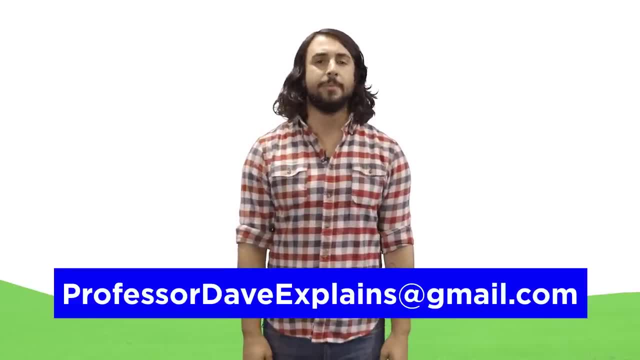 Subscribe to my channel for more tutorials and, as always, feel free to email me professordaveexplains at gmailcom. I'll see you next time. Bye-bye. 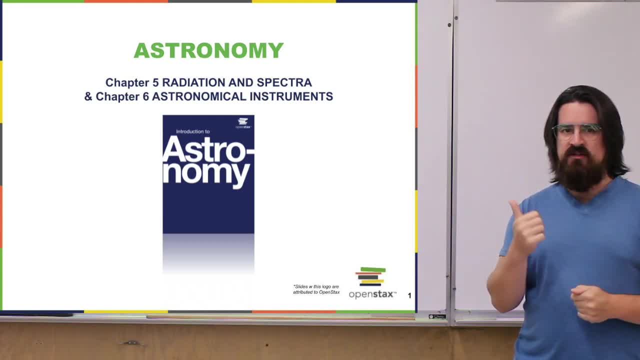 Here we are again, lecture number two about astronomy- descriptive astronomy. This lecture is going to cover most of the material in chapter five and six of the text And, in short, that's about the kind of stuff that astronomy looks at, uses to analyze.